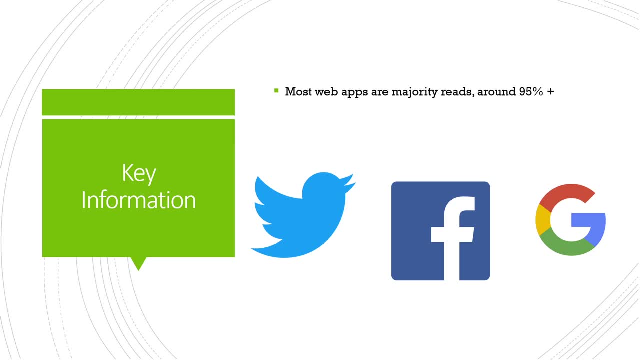 out how to scale your database is that most web apps and applications in general are very read heavy. It's usually around 95% and, if you think about that, something like Twitter, one large account. they write once to the database to create a tweet, but that one tweet can be read and retrieved from the database millions of times. 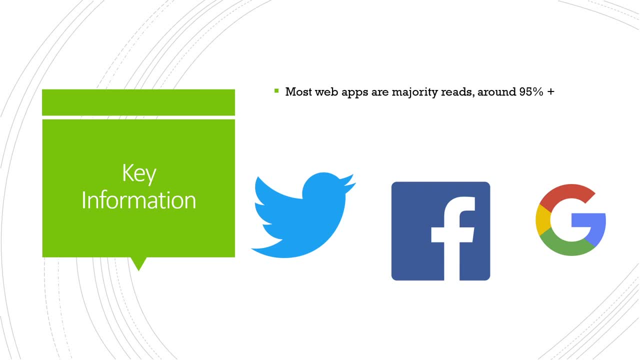 Same thing for Facebook with posts on there, and Google, when they index a piece of information, that the metadata that web page isn't going to change very frequently, but a lot of people are going to be making searches for those web pages. So in almost all cases you're going to want to. 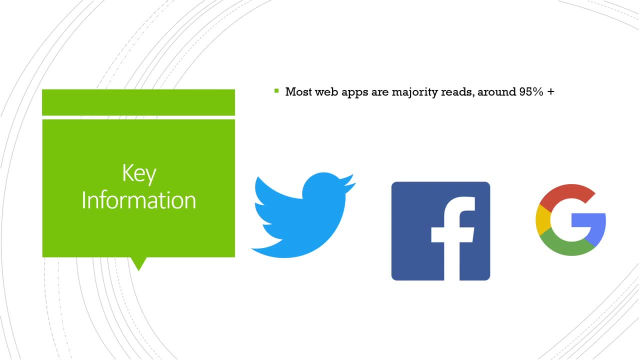 prioritize and build around the idea that your databases are going to be receiving a lot more reads than writes. So these are the simplest ways to start off when trying to improve the performance of your database, and I'll just go over them one by one, So the easiest is obviously. 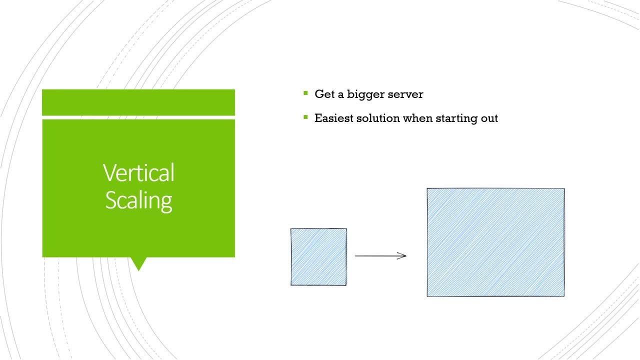 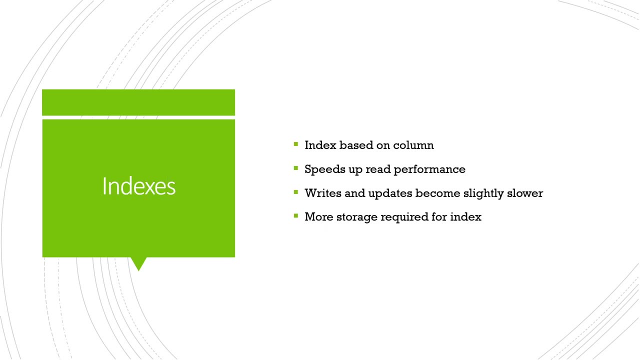 vertical scaling. you don't have to change anything. you literally just move your database to a bigger server, so it has a faster processor or more memory. You then have indexes, so what happens with this is that you create an index based on a certain column that's frequently accessed, so it 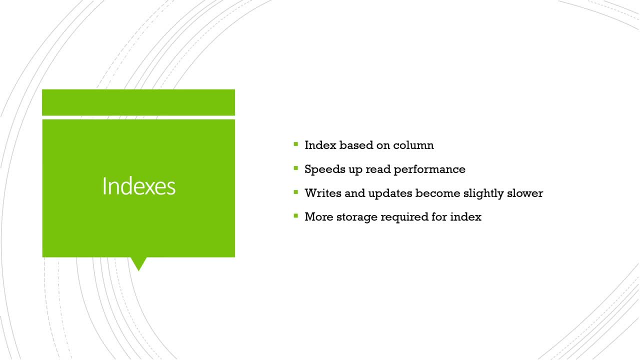 could be something like the user id or something like that. It speeds up read performance by creating an index that speeds up the lookup, so it doesn't have to do full table scans across your database. The downside is that writes and updates become slightly slower, and that's because 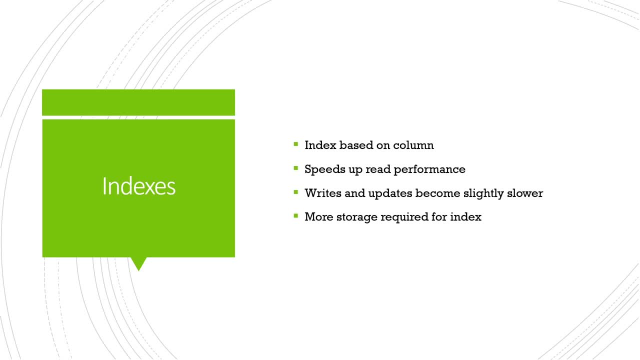 every time you update a row, you also have to potentially modify the index And you also require more storage for a table that's indexed, because you have to store the index itself. Denormalization is where you actually go against a standard best practice with relational databases and you add redundant data to tables so that it reduces the amount of. 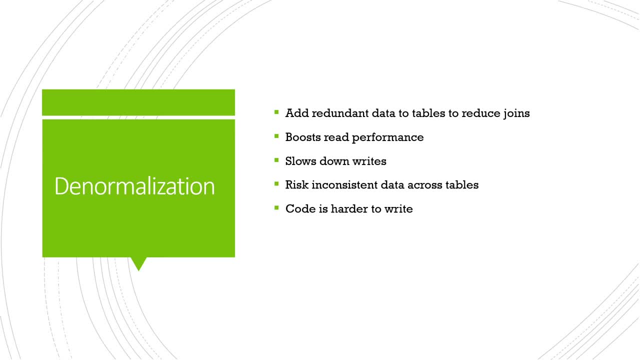 joins you need to do, which improves your read performance. A downside is, once again we're sacrificing write performance and we're risking inconsistent data across tables, because if you have something that, let's say, it's in two tables, now you have to somehow figure out a way so that those values, when you write to one table, it also changes that data. 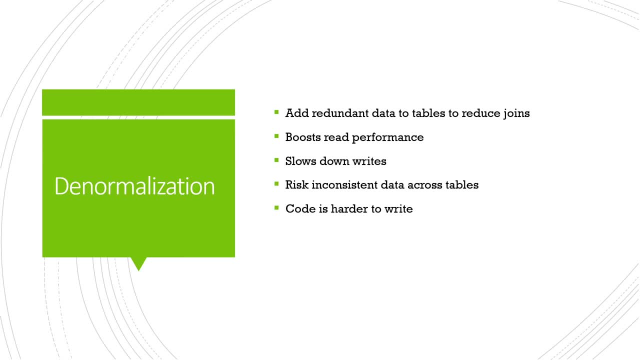 in the second table, where the data is also located. Otherwise you could get a situation where somebody tries to retrieve the data and the value is actually different in two different places. so you then have inconsistency, which for certain applications could be a major issue, The other 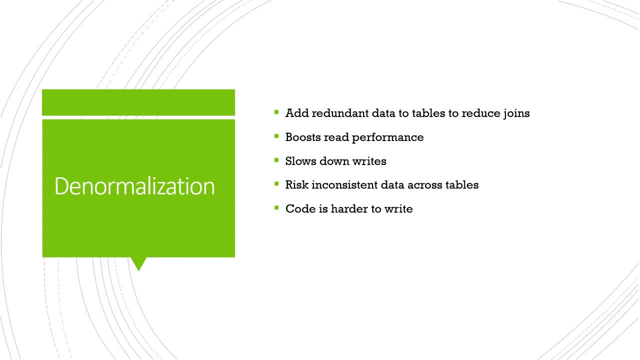 factor is that the code becomes harder to write because you have to deal with that situation where you're not only writing to one table but you have to update that data in every place that that column is now located. Usually that's abstracted away by some sort of library, but 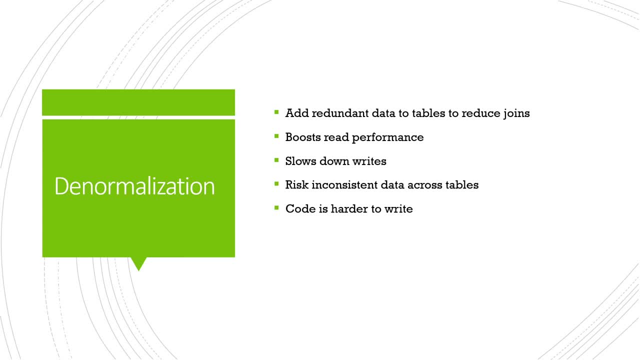 obviously somebody has to create that library to handle that Connection. pooling is a pretty simple thing to do. Kind of a metaphor or a way to think about it is. it's like carpooling, where everybody just rides in the same car to save money. You have aarm to be able to do that same way and the rest of your 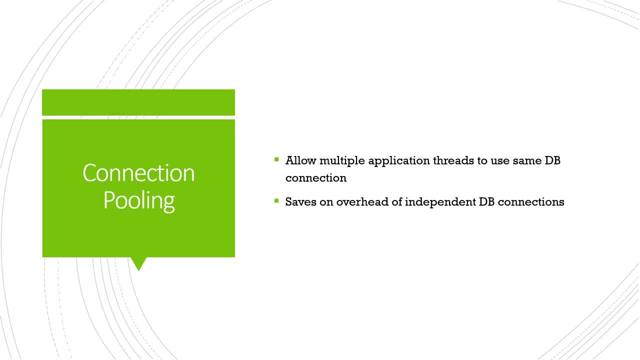 to save resources or save money. in this case, what happened? what's happening is that instead of every application thread using its own connection, they're pulled together and kind of use the same one, so it saves on overhead of independent connections to your database, one of the most important ways to scaling your 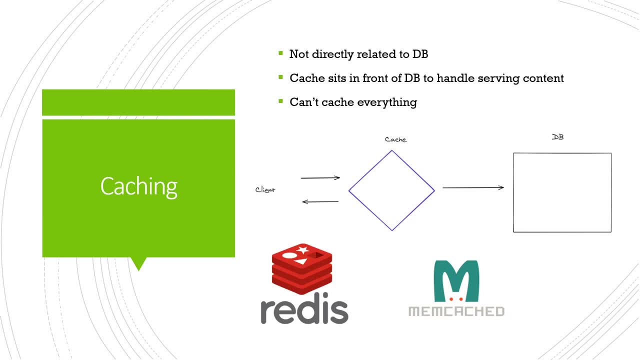 database server is actually not directly related to the database at all. it's called caching, and what the cache does is: it sits in front of your database and it can serve traffic from memory rather than having to read from disk, and what this does is drastically improve performance. so, for example, on a, you have 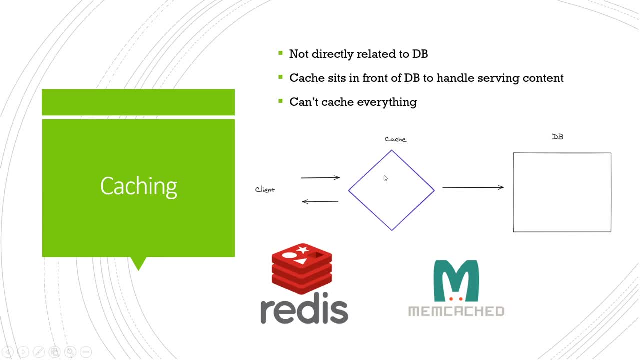 a client requesting data. for the first request it would have to pass through the cache because it's not located there and get it from the database. but then the database or the cache would store that result and for any subsequent requirements the cache would serve that directly and it's basically the best way of scaling. 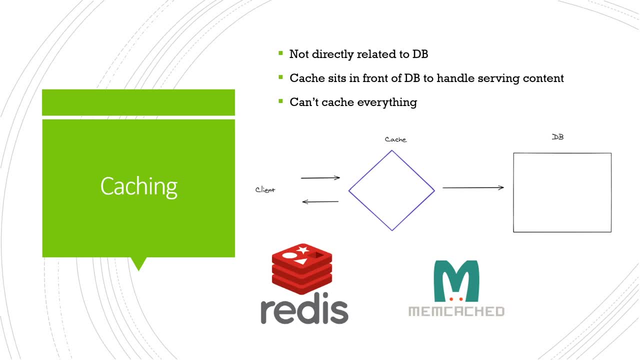 your database is to not let traffic reach your database at all. and cache because if you're familiar with the difference between, like random access memory RAM, it's much faster than reading it off of whatever storage you're using- Facebook, for example- it's pretty much the most important part of their 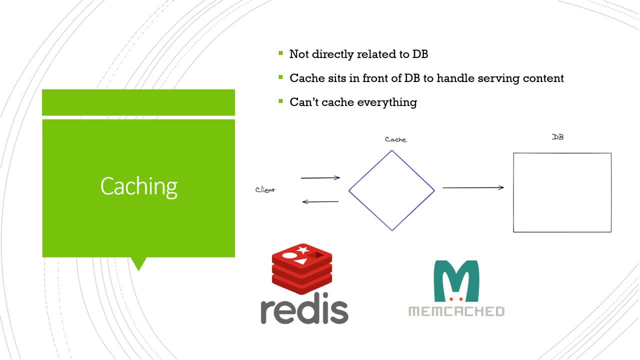 infrastructure. they released a paper about caching in 2013 that said about 99% of their requests are served from cache and it's pretty much the most important part of their system, because anytime their cache servers went down, the databases could just couldn't handle all that traffic hitting them. so their 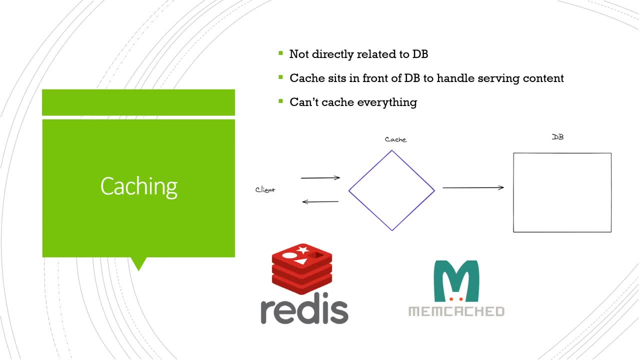 entire goal of engineering is basically to protect their databases from all that traffic using their cache. the only real issue with caching is that you can't use everything with the cache, so you can't use everything with the cache, so you can't do everything. you want to change anything with caching because it is. 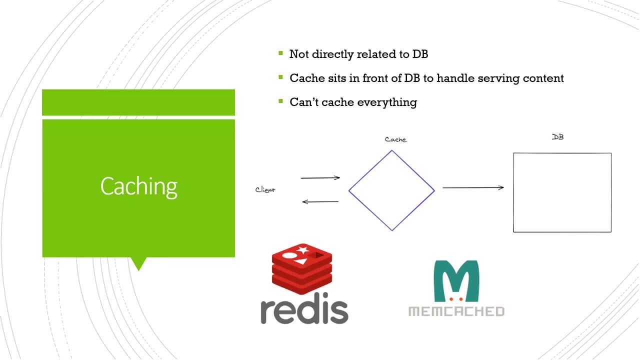 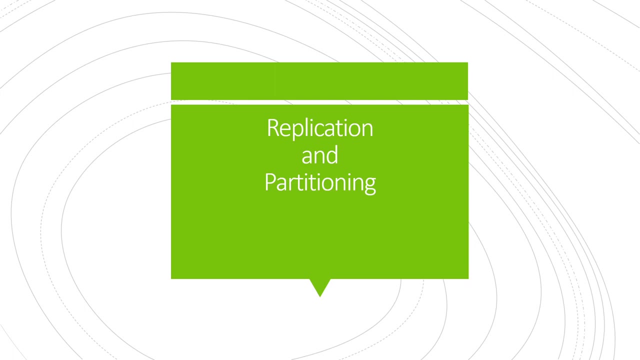 just you, and now you have to switch to the compute method that you just need if you're using caches, right, so that would be the best way you can launch caches through don'tersport or right now in Adobe Cache. okay, they're lacking something, obviously, if you install apps on your cached database. 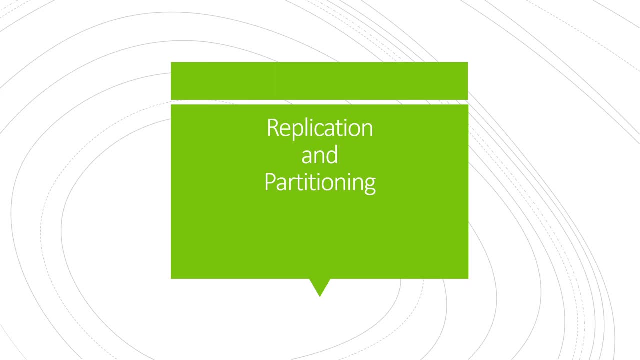 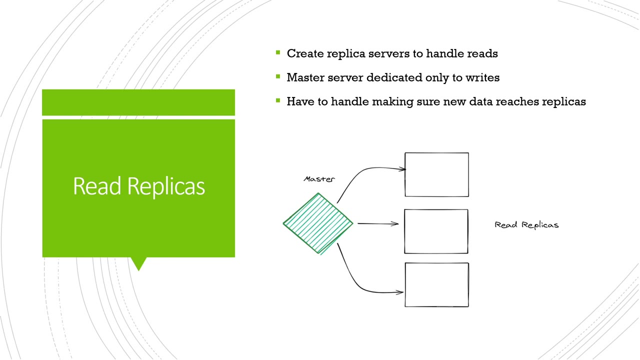 you should be able to access them and they'll apply and request the hard governance that you need, but not everything they need to do, for example, on macrosoft document landing back що that they don't need to use. so it's a good going to be read replicas and the way this works is that you essentially duplicate your databases. 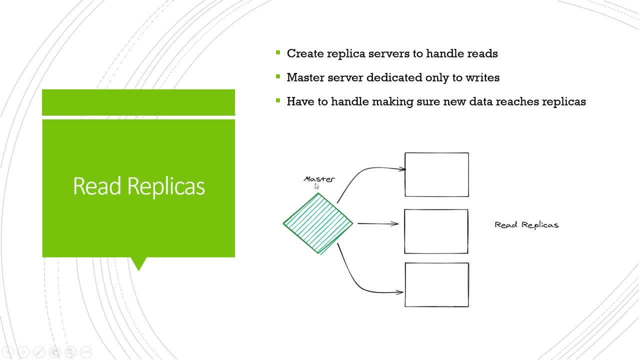 and you have what's called a master. this will handle all new incoming write data and then you have replicas that handle anything requesting data. these handle it. to take um, take traffic load off this master. the issues that come in with this are that you run into consistency issues, so 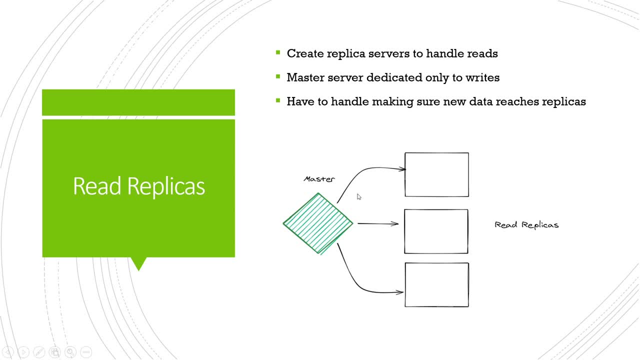 let's say something goes wrong in your data center. this connection between the master and the replica is broken and now you have client requests coming in and this, because it's not being updated, will have stale data. so, depending on your application, that could cause big issues. it could frustrate users because they're seeing the same stuff, they're not getting access. 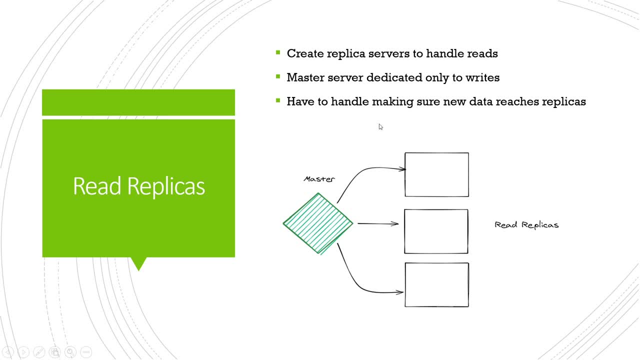 to the newest data or the most recent data, and that involves to take care of that problem. you have to do a put a lot of engineering effort to handling, detecting when a database is down, bring it back up, rerouting traffic to your other databases. a side benefit of this, though, is that 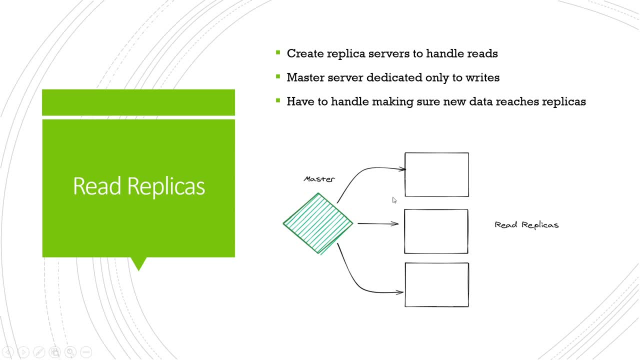 you have built-in fault tolerance because, like i said, if one of these goes down, you no longer have just a single database handling everything. so even if one of these goes down, you still have these backups. so an additional benefit and to handling more traffic is that you also have fault tolerance. 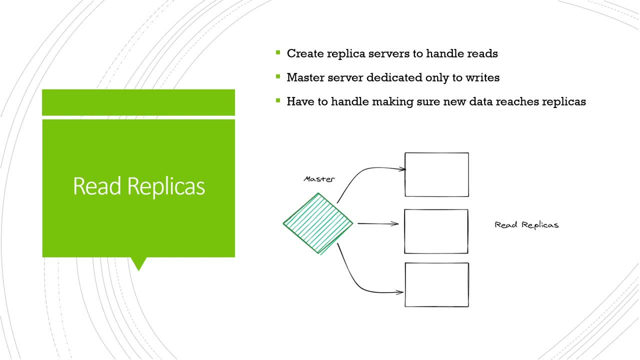 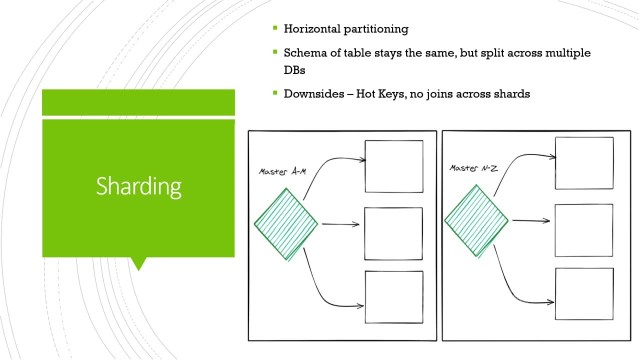 in the case of some sort of error. now we move on to partitioning, and the first type, which you probably heard about, is called sharding. so this is horizontal partitioning, where the schema of your table stays the same but it's not split across multiple databases. the big reason for this would be if your read replica set up you. 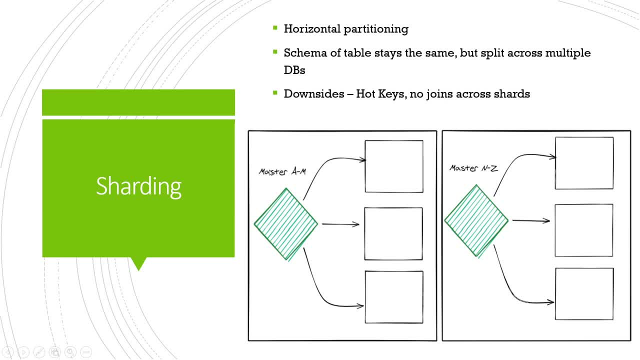 need to handle more rights, so you split this up. so this case, we'd be doing it by like name of the user, so you have letters a through m. people's names a through m are stored on this shard, and this one, n through z, is stored here. the big upside, of course, is that you can now handle more. 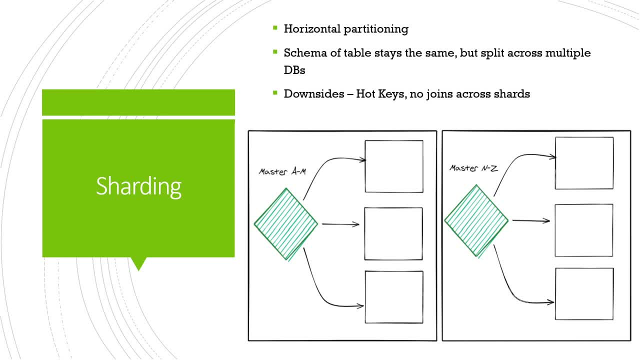 traffic. the downside is what's called hotkeys, so let's say, like xyz, those names aren't going to have as much traffic as certain other letters, so it can result in uneven traffic. if you're not careful about how you're sharding your database, you also have issues that you can't join across. 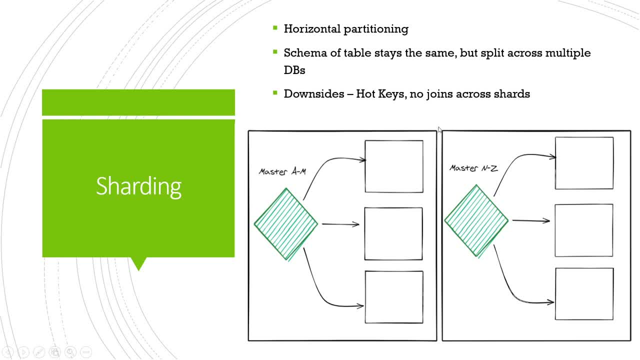 these shards because the data is separate. if you do, it's going to be very slow. a famous example like a hotkey issue was instagram. they talked about it with justin bieber, so his name or his user id had way more traffic than the average user and there's really no good way to handle. whenever he'd post a picture, their servers 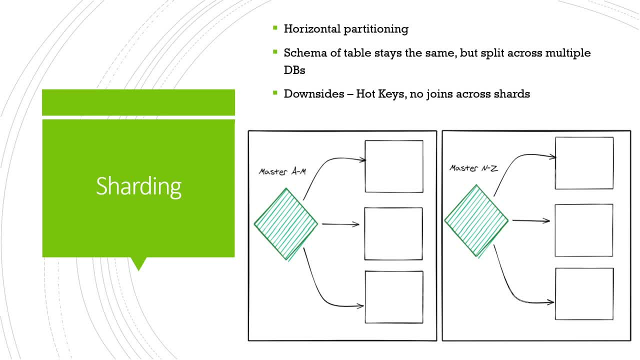 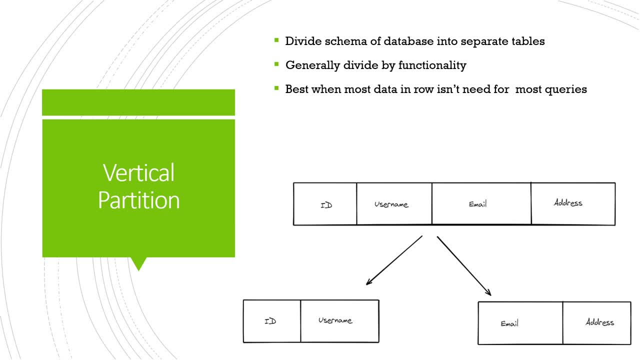 would go crazy. so that's in some cases. there's really no good way to actually handle sharding. you just have to kind of deal with it. so sharding was horizontal partitioning. you also have the option of a vertical partition, so in this case you're actually dividing up the schema, or schema of your database into separate tables. 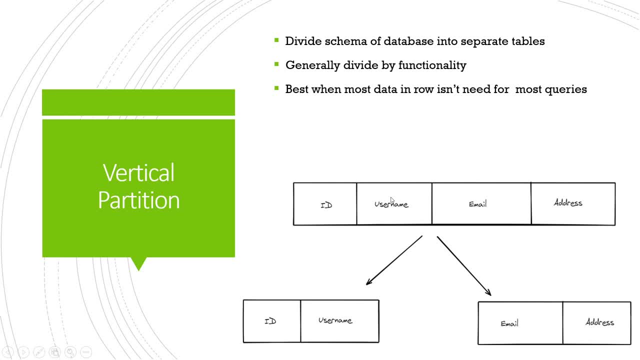 typically that would be done by functionality. if you have one big row of user data and you realize looking at your analytics that in some cases, certain amounts, they're not really used together, it would make sense to split those apart so that you're not retrieving um a bunch of extra data you don't need. and also it would reduce the size of each database because 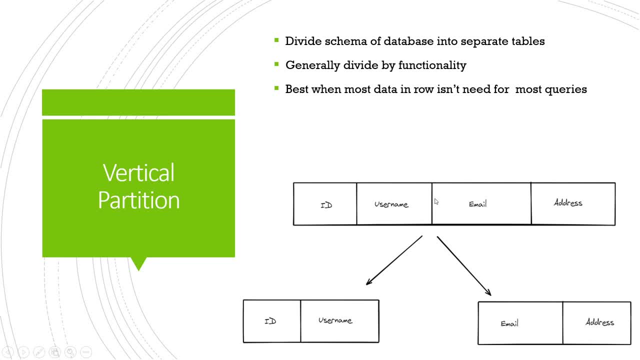 you're essentially, in this case, splitting it in half. examples of this is, once again, instagram. in their case, they actually completely split off the light counts for photos from everything else, so it has its own custom data store so they can have the performance they want for light counts on a user's photos. 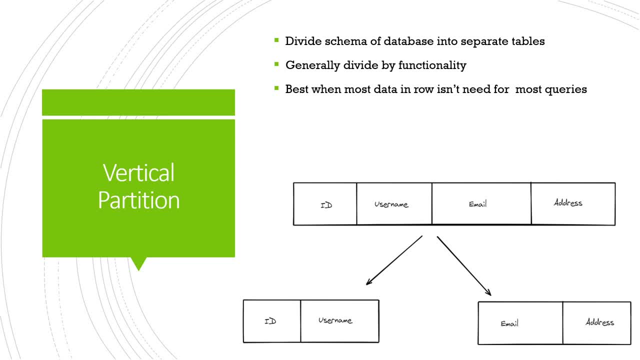 so that you can easily share them to your users. so this is a very similar way of doing this, but you can also do this by using this as a way of doing this with other programs in the same way. so this is sort of a general concept of what's called sharding. 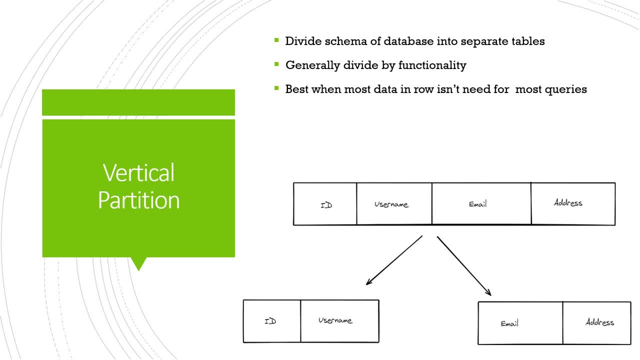 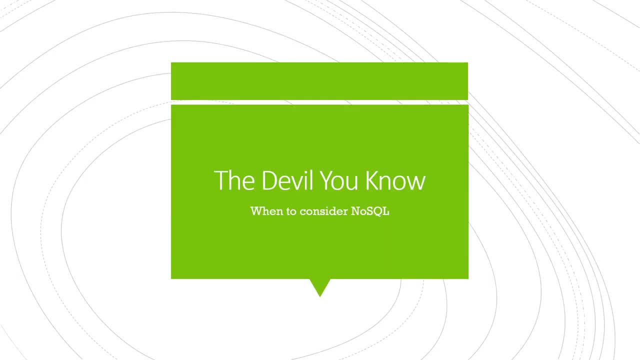 and that's the way that it's implemented, in the form of sharding. generally, this is easier to implement than sharding, but the downside is that you could potentially end up having to shard or horizontally partition anyway, and then it can get really complicated because you've already vertically partitioned and now you 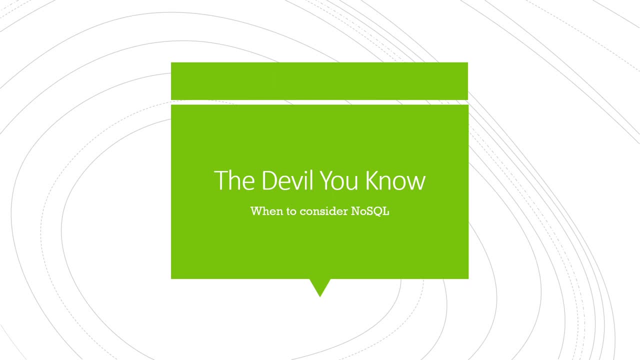 normalized data is gone. strong consistency is gone. a simple data model is also gone. so we've made so many trade-offs trying to scale this that it's almost unrecognizable compared to a standard sql stand setup. in this case it's one you might consider some sort of no sql database. 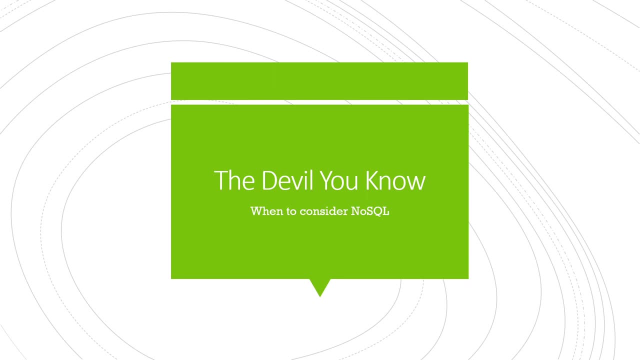 the thing to keep in mind is the reason you choose. this isn't because no sql or no sql is magical. it's the fact that up front, you know what you're sacrificing. when you started off with a relational database, you kind of thought you'd stay with all the best practices. 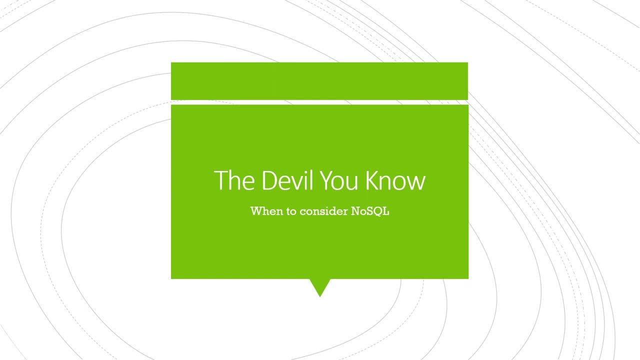 and by the time you've ended up scaling, you've already lost all that. so the reason you choose a no sql database is that you know exactly what you're going to be sacrificing. you know what specifically you need for your application that you can make a trade-off. 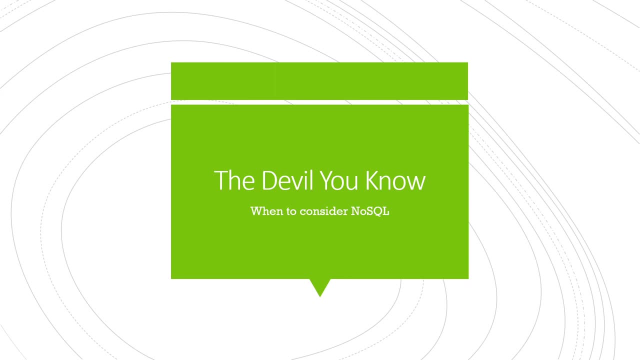 so if you're doing something with like transactions and banking, you obviously want consistency. but for stuff like google or social media, where you don't need perfect consistency right away, you could make those trade-offs for scale. so it's kind of the devil, you know, with s, with no sql. 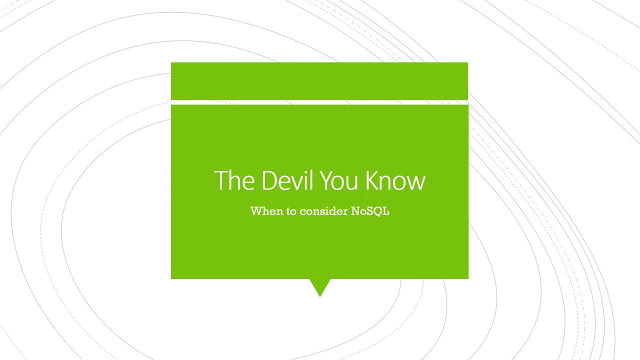 you up front are making the choice and that way you don't have any surprises down the road. with that said, i'll be going over in depth no sql versus sql databases or relational databases in a future video, so be sure to subscribe if you're interested in that. if this helped you out, hit like it helps.